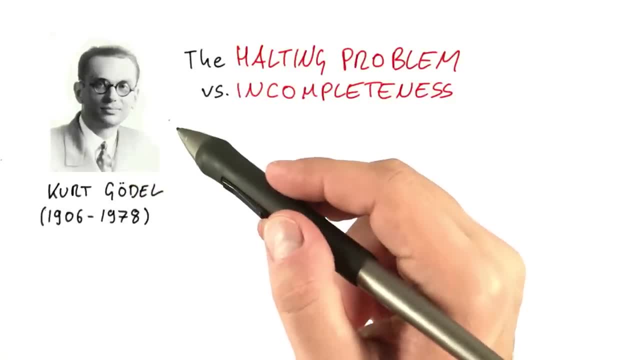 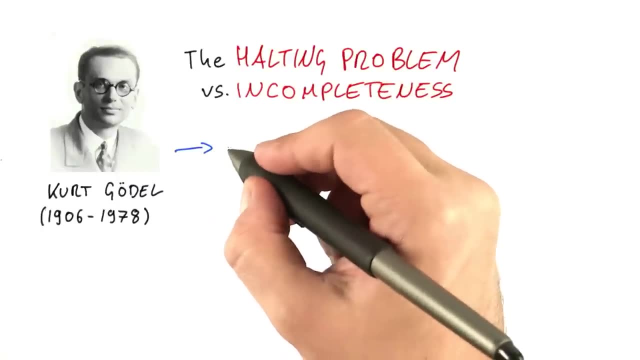 mathematician Kurt Gödel, are concerned with mathematics but are actually closely related to undecidability And, as you might know, any mathematical system starts out with a set of axioms. What are axioms? Axioms are statements which you assume to be true without having any. 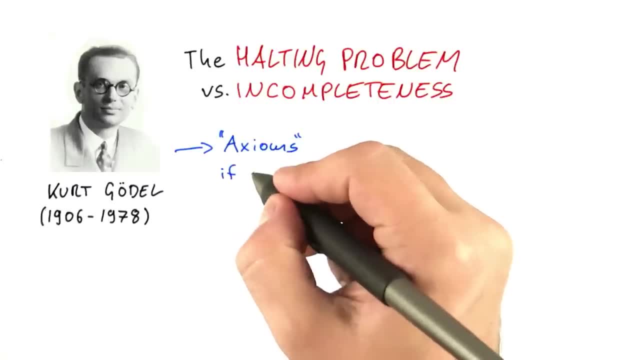 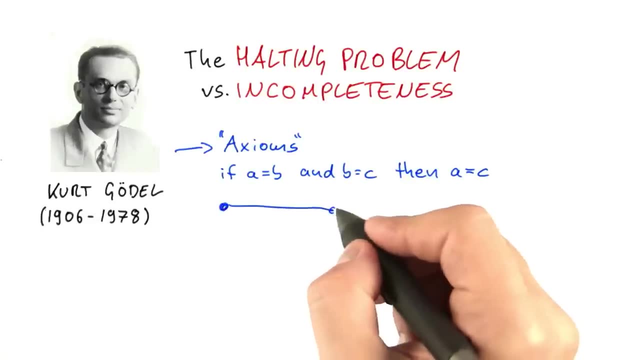 formal proof for them, such as: if A equals B and B equals C, then A must also equal C, Or you can always draw a line from one point to another point, no matter where they are. Those would be axioms. Now, axioms often sound very trivial, like this one here, or the fact that you can always 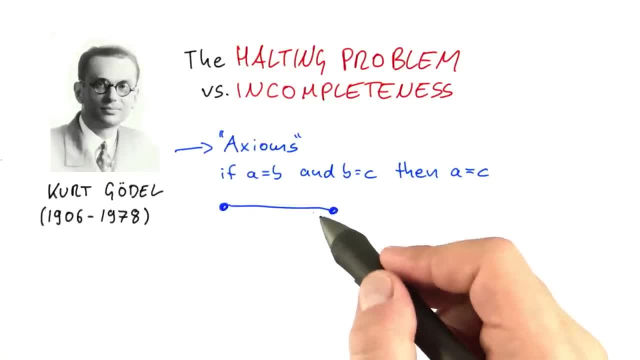 draw a line between two points, But for many of them there are actually scenarios where they are not true. So axioms are the basis of mathematical theorems and axioms are the basis of mathematical theorem or proof. Now what Kurt Gödel showed, and it was a shocker at his time and to many- 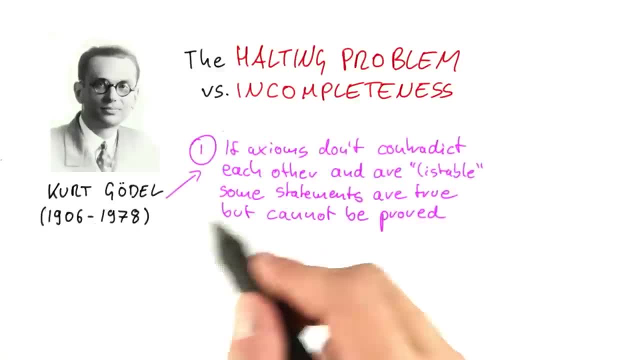 it is still today- is the following: So what Kurt Gödel showed was that if you have a set of axioms and they don't contradict each other and they are listable, which means you could have an algorithm that lists you all of these axioms, So either they are finite or they can even be. 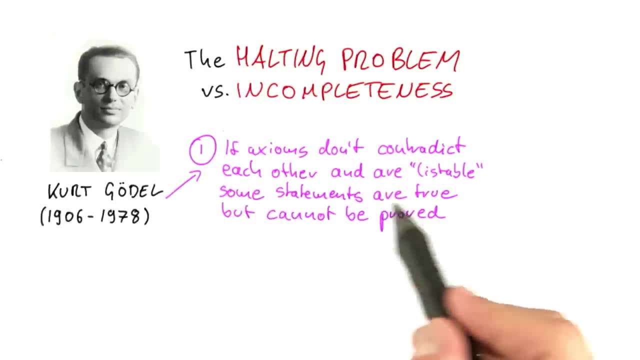 infinite as long as you have an algorithm that can produce them all. If this is the case, then there are some statements that are true but which you cannot prove based on the fact that they are based on these axioms, And this is what he meant by incompleteness. So he basically showed that. 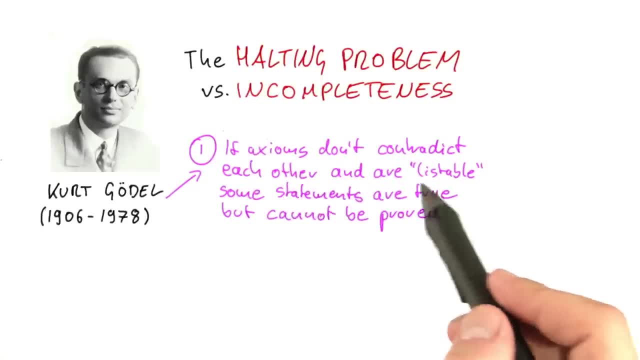 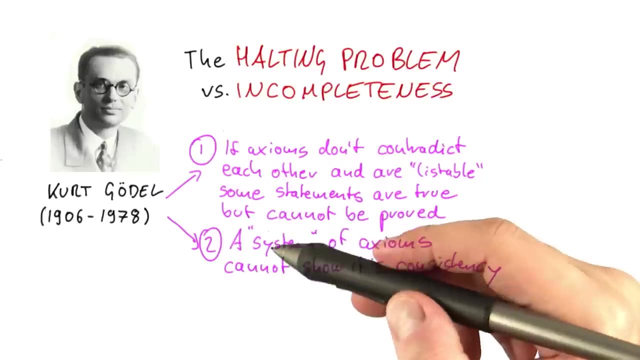 no matter what foundation you base a mathematical system on, as long as that is a consistent foundation, then you cannot prove everything without adding additional axioms at least. And he also showed- and this is the second incompleteness theorem, which is basically an extension of the first one- that a system of axioms cannot demonstrate. 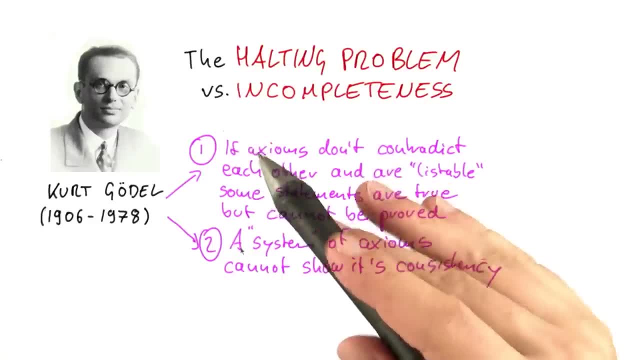 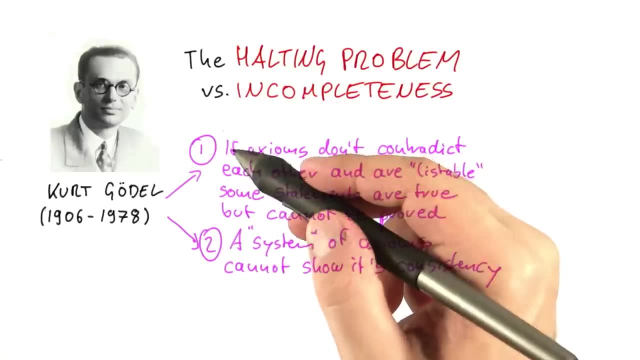 its own consistency, And what that means is that, very informally, a mathematical system cannot be used to show that it itself is consistent. And these two statements are, in a way, very similar to the halting problem and undecidability. 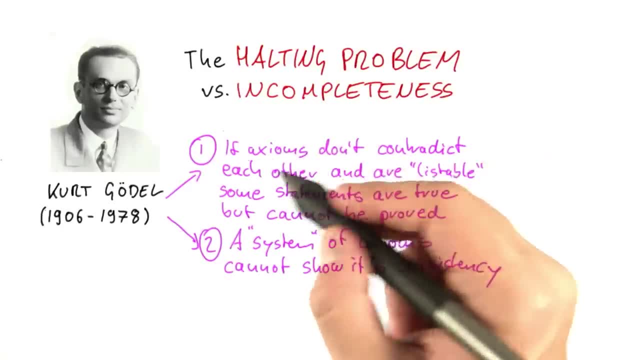 The axioms. you could think of those as programming statements. So any program or algorithm is composed of a number of simple instructions that are then arranged, And of course there's an infinite number of possible computer programs that you can write. but they are made up of a finite set of building blocks. And the second incompleteness theorem.